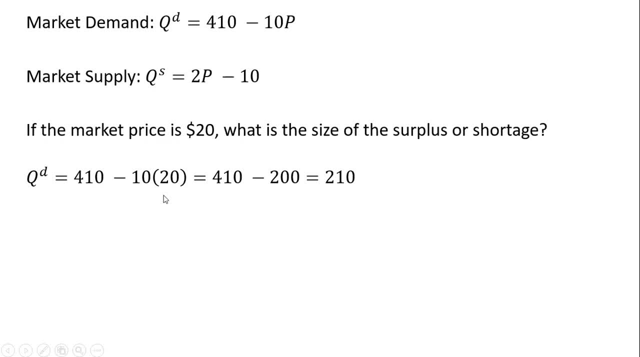 the math here, We're going to get 410 minus 10 times 20, or 410 minus 200.. So we have a quantity demanded of 210 units At $20,. consumers are willing and able to buy 210 units. Let's see what. 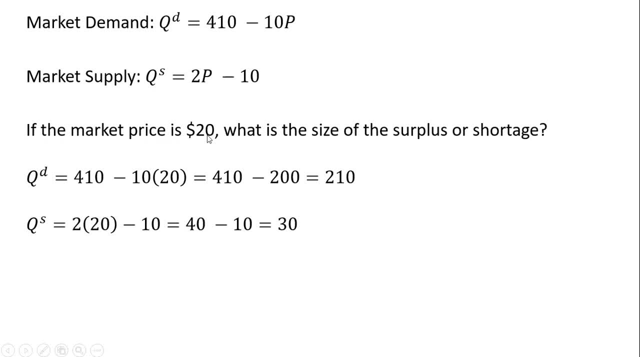 happens. on the next question: If the market price is currently $20, what is the size of the surplus on the supply side? Taking that same $20 and plugging it into the market supply, we see that sellers are willing to bring 30 units to the market. 2 times 20 minus 10 is 40 minus 10, or 30. 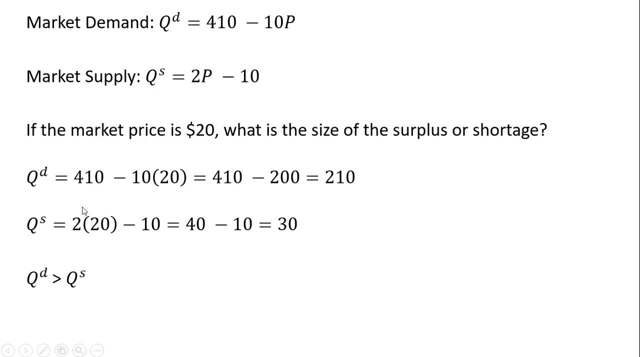 units In this example, then the amount that consumers want to buy exceeds the amount that sellers want to produce and offer for sale. This is the classic example of a shortage or excess demand. Quantity demand is the same as quantity demand, So if the market price is currently $20,. 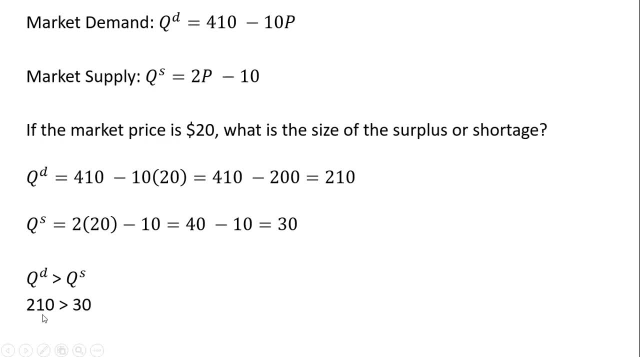 it exceeds quantity supplied. 210 is greater than 30.. We can calculate the size of the shortage. Consumers are only going to be able to buy 30 units. They would like to buy 180 more. so that is going to be the shortage. 210 minus 30 means that there's consumers out there that 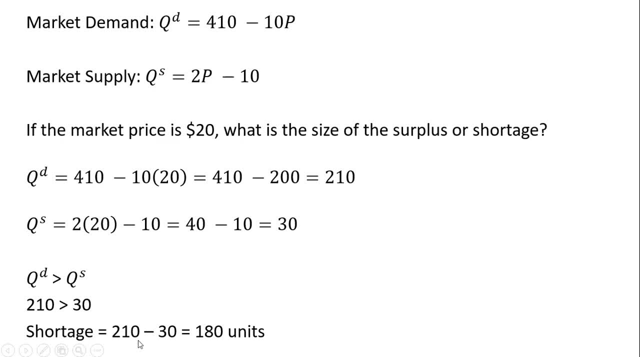 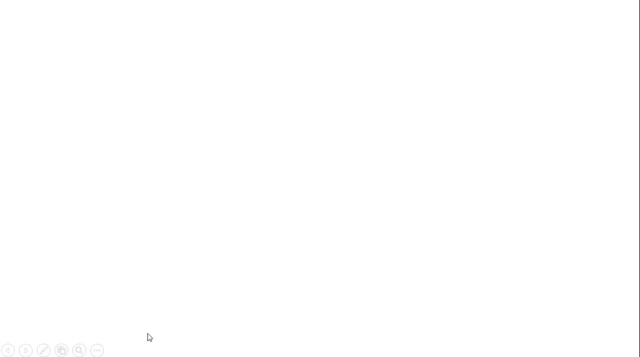 would like to buy 180 more units and is currently being made available by sellers. All right, let's move on. Same market demand, same market supply. Let's try now a market price of $30 and see what happens. So again the same idea. We're going to plug this $30 back into the demand. 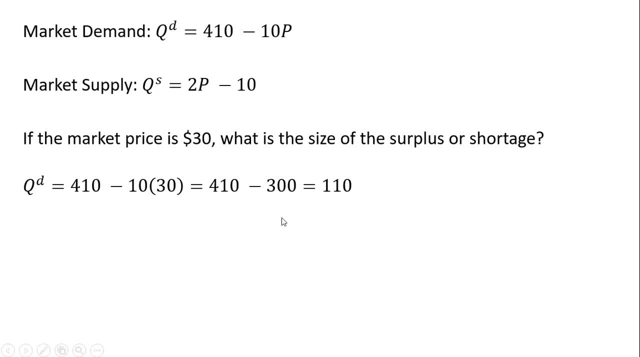 and supply equation, Plugging that into the demand equation. consumers would like to buy 110 units. Sellers with the higher price would like to bring a few more units to the market. here, they'd like to bring 50 units to the market. nevertheless, we still have a.